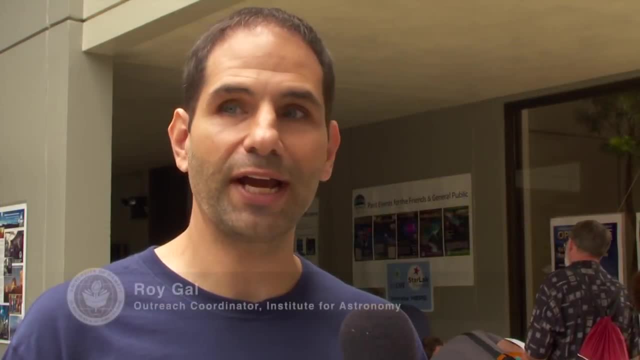 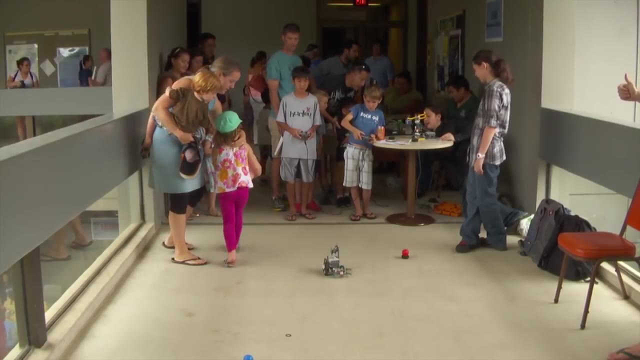 has two goals. One is to get the community to know that UH has this incredible astronomy institute right here in everyone's backyard, And the other is to get kids interested in STEM fields- science, technology, engineering and math- and show them it's not just equations and 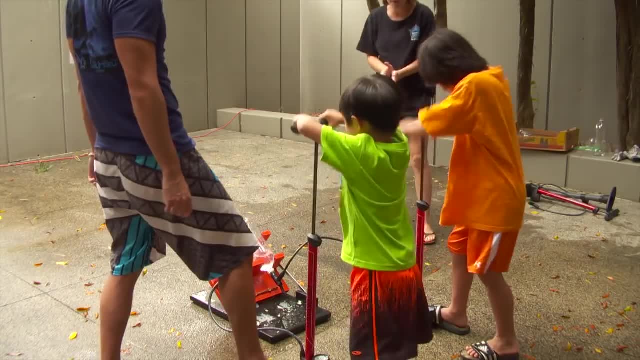 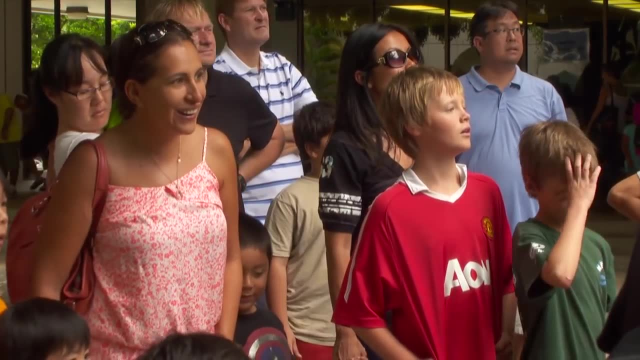 boring, but actually a lot of fun and a lot of cool things going on. The more than two dozen exhibits and activities are designed to give kids of all ages and adults a hands-on experience in astronomy. We were putting air into the bottles with water. 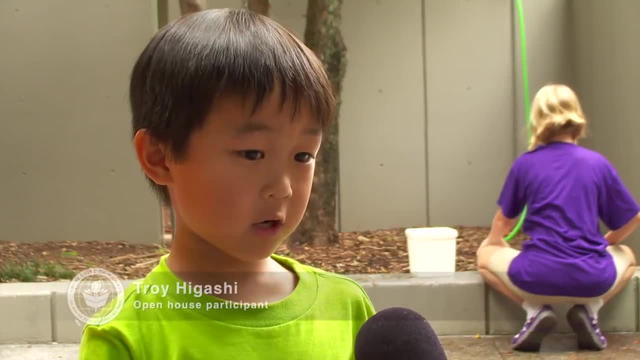 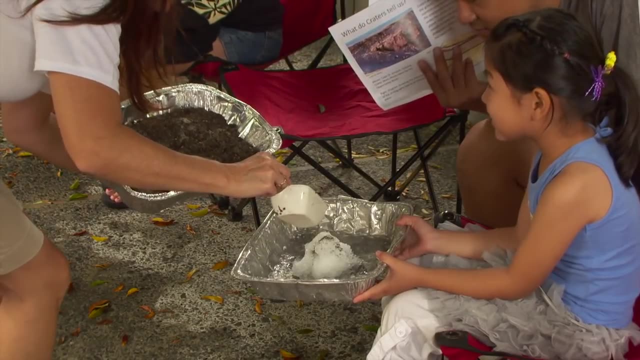 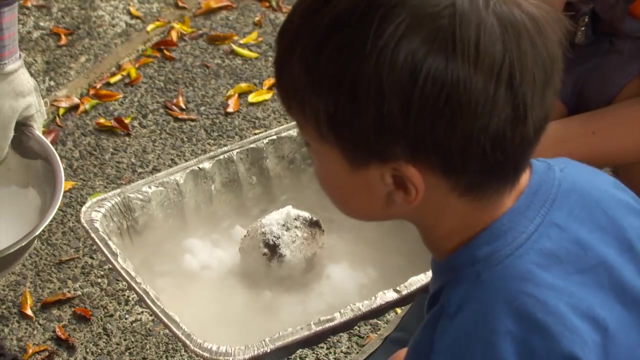 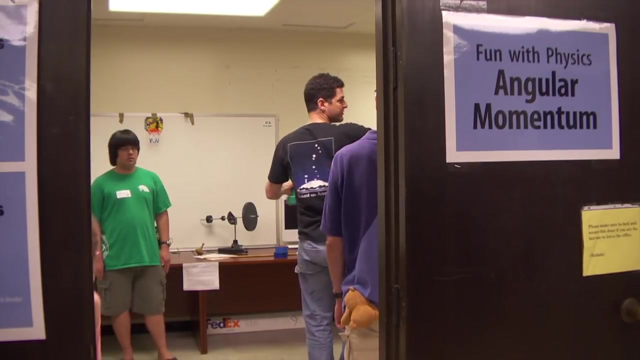 We're going to make our own comets, and we made our own like a snow bar and then dirt and sand over it. The open house, which averages about 1,300 people a year, gives UH educators and students a chance to share their knowledge and passion for astronomy and science. 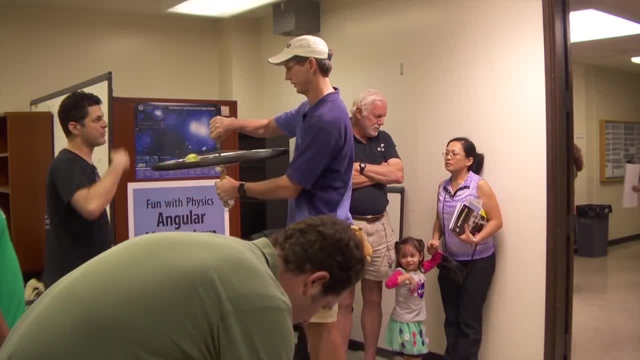 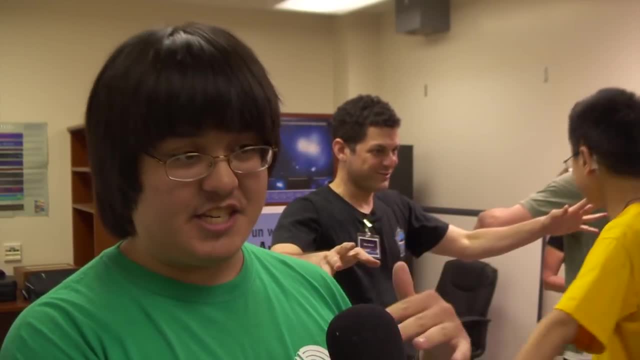 We're just doing a whole bunch of demos about angular momentum. It does everything, from your bike stays up while you're riding it, all the way to making sure the galaxy keeps its shape. There are also talks and presentations by faculty and researchers, who are among the 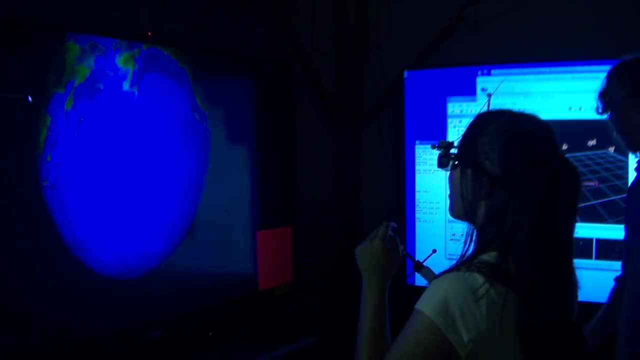 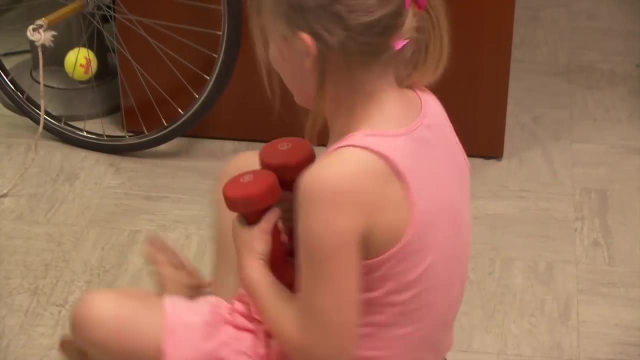 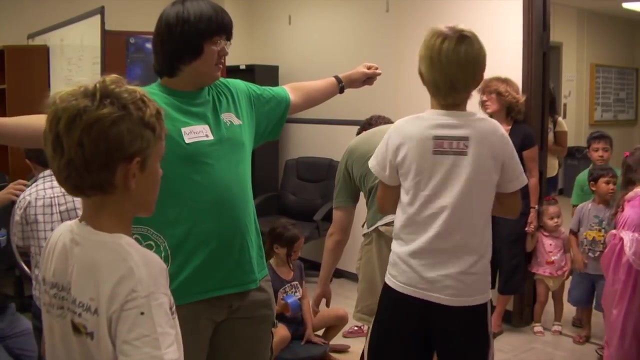 best in their fields, along with movies, stargazing and the exhibits and activities, all presented in a way that makes learning about astronomy fun. Everything from the theory to the experts to the practice. You get the whole experience From an internationally recognized 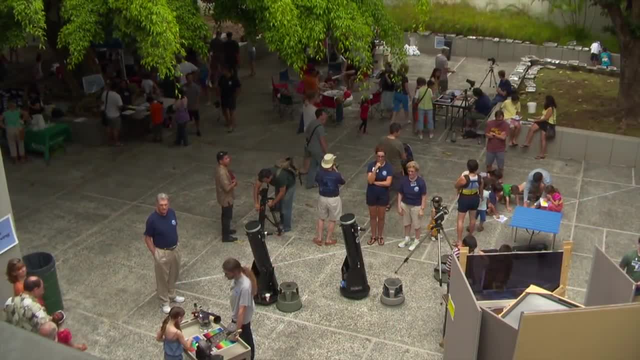 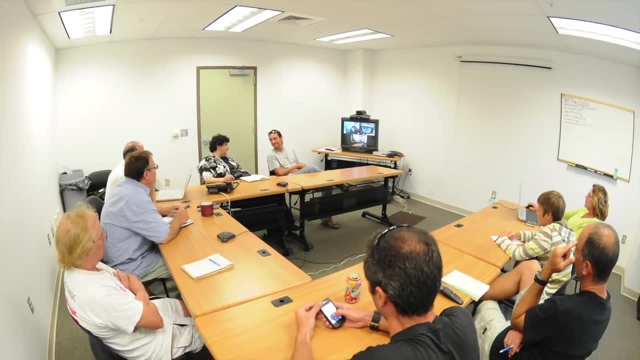 department. It is the largest university astronomy department in the country that brings in an average of $20 million a year in research funds from outside the state. It attracts the top minds in the field, performing a wide variety of research. thanks to UH's access to all the 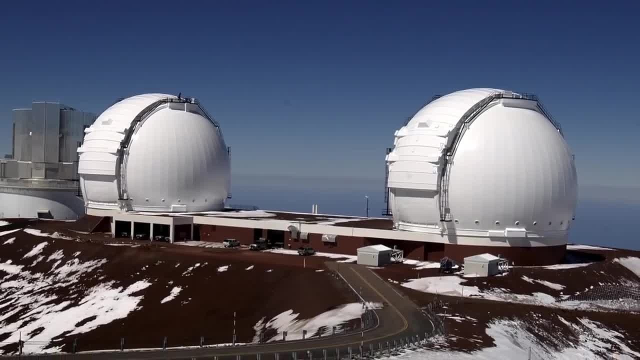 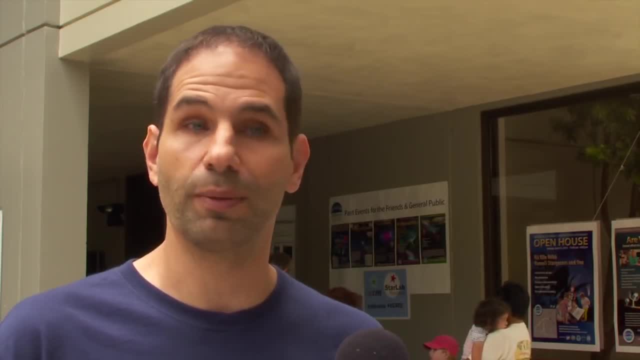 telescopes on Haleakalā and Mount Akaia. We have hundreds of kids going through our intro astronomy classes who get to use our telescopes here. So we produce great PhD students going on to some of the best careers in astronomy out there. 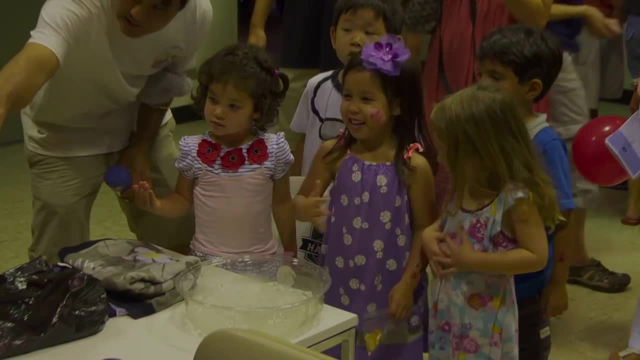 Chances are, you will find some of those future PhD candidates at the Institute for Astronomy Open House each year.